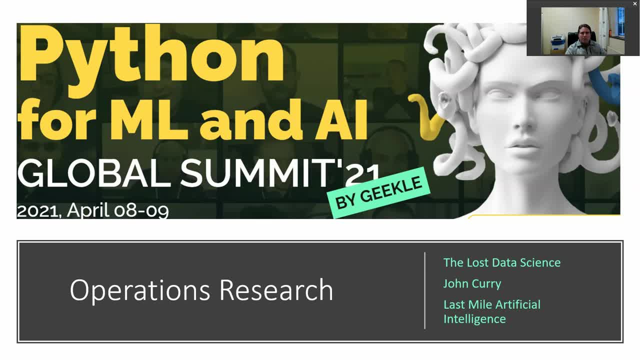 Hi and welcome to this talk on operations research, the lost data science. I have to admit that I'm taking some poetic license with the title, but I hope to convince you that it is in fact accurate in many ways, OR is something that is lost, to us at least. 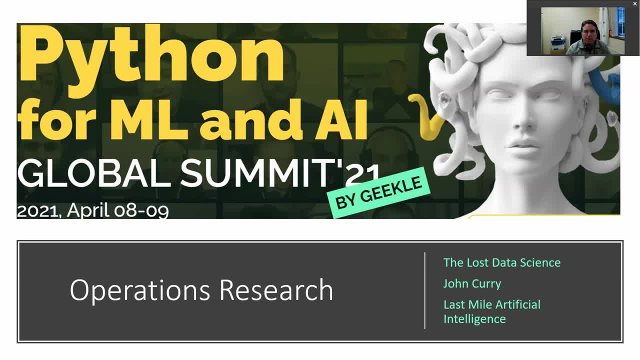 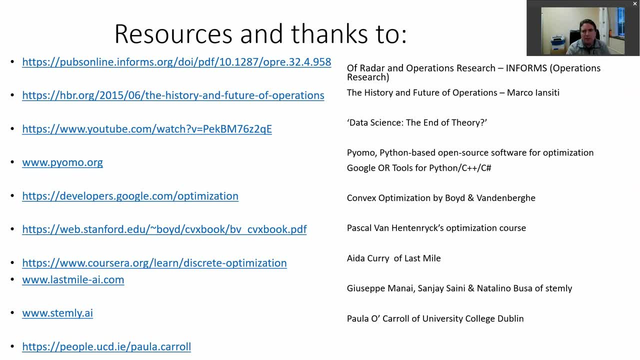 in the Python AI community and it needs to be refound. Thanks to Ida and the Last Mile crew, Giuseppe and the crew at Stemley and Paula O'Carroll of University College Dublin for reviewing this work. all mistakes and outlandish claims. 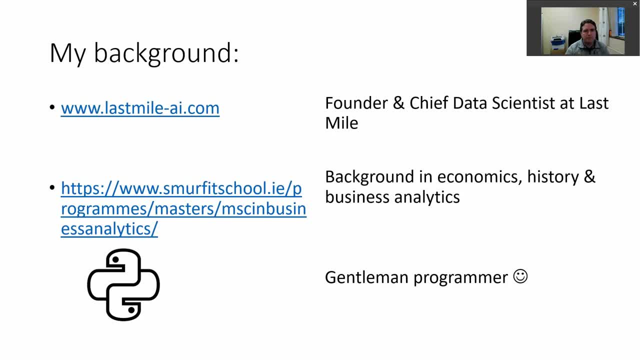 are entirely way on, So you may have heard of the phrase gentleman farmer, a somewhat disparaging description of someone who merely dabbles in farming. I jokingly refer to myself as a gentleman programmer. My main job is collaborative problem solving using whatever conceptual and technical. 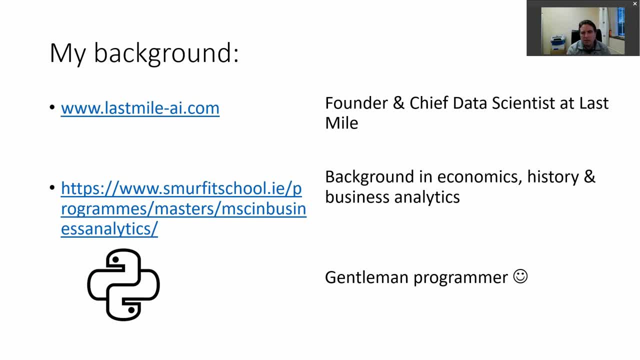 tools I need. I manage a team, but I find that working hands-on gives me ideas and tests those ideas. I do program a fair bit and I'm keen to learn more Python for ML at the conference. What is my motivation for the talk? Well, I was lucky enough to take combinatorial optimization. 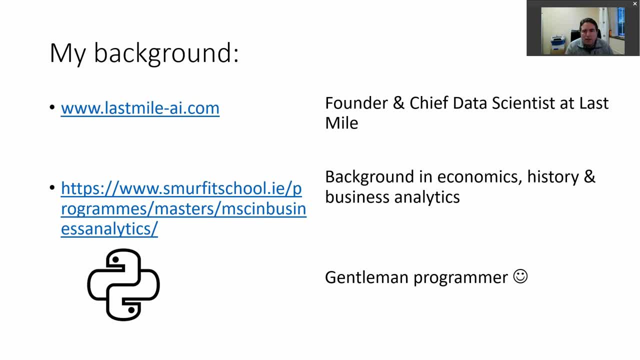 when I studied business analytics in University College Dublin. It's not in the curriculum for most computer science or data science degrees. On several occasions over the last decade I've seen senior data scientists with PhDs fail to solve some major business problems. Each tried using machine learning, graph analysis or other standard tricks-of-the-trade. 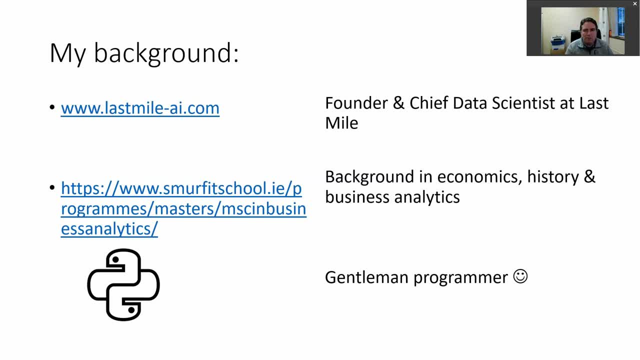 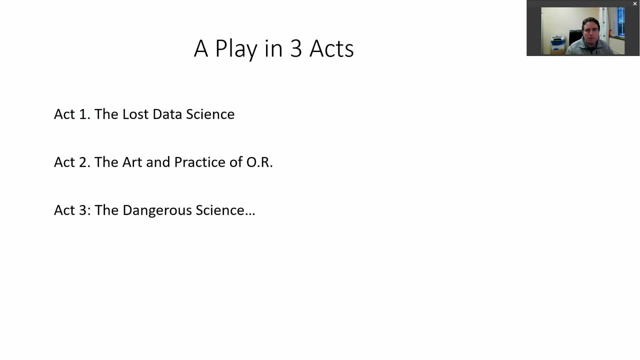 In each case they failed and in each case the problem was clearly solvable as a combinatorial optimization. You only have a hammer. everything looks like a nail. So let's see what the field of OR should mean to us as working data scientists. 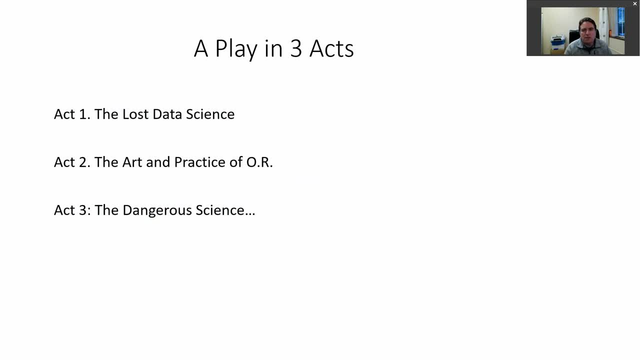 First we'll explore OR why it is somehow lost to data science and why it needs to be found. In Act 2, we'll find out how OR fosters design in mathematical thinking. I'll give you some pointers to get started on optimization in Python. 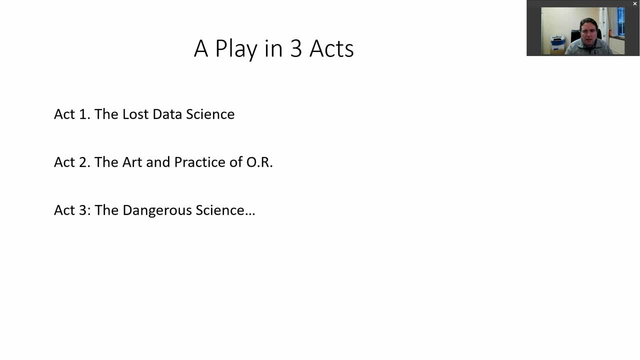 And finally, in Act 3, how? OR gives us transparent AI and actually increases the number of ethical problems we're going to face. So when we solve a juicy problem, we're always faced with the next one. This is no exception. So the lost data science. 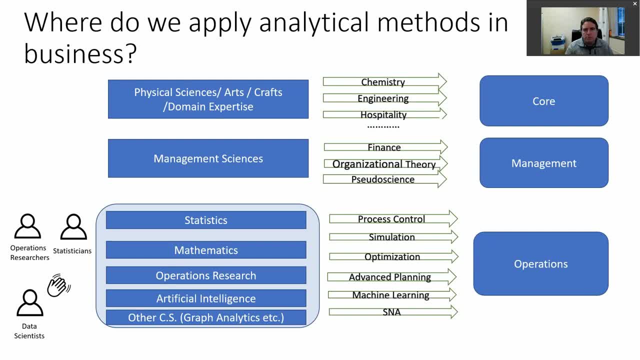 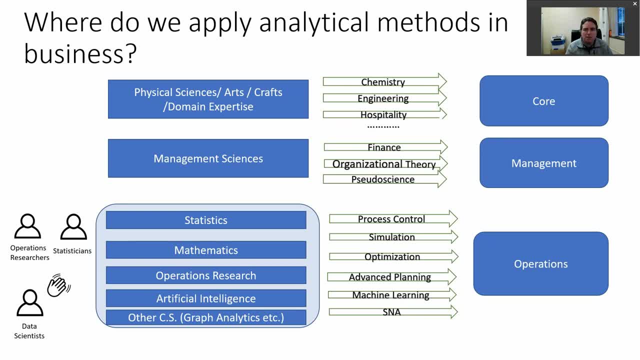 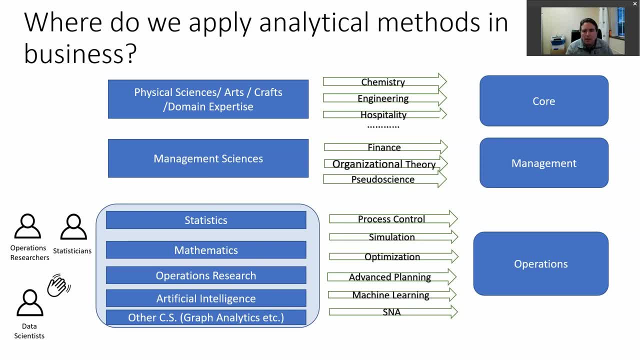 It's the traditional R&D that drives economic progress. At the management level it will be some useful methods around financial planning, and the less said about the rest, the better. It's the operations level that really interest us. as data scientists, We make things work. 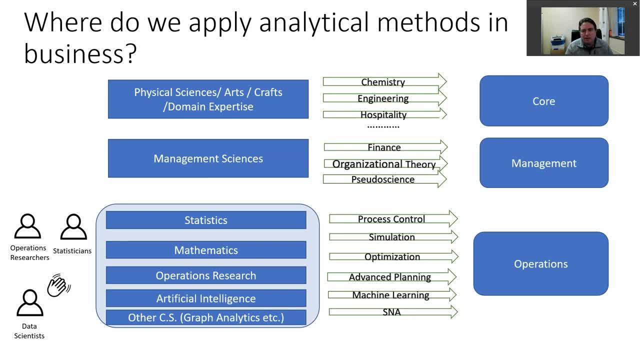 We make things work. The problem here is how to apply analytical techniques to operational data to understand the business and improve outcomes. Although data science is cross-disciplinary, essential techniques these days are from machine learning coming out of the AI labs or CS departments. 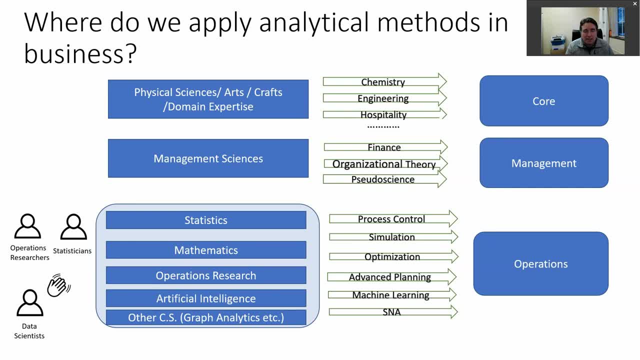 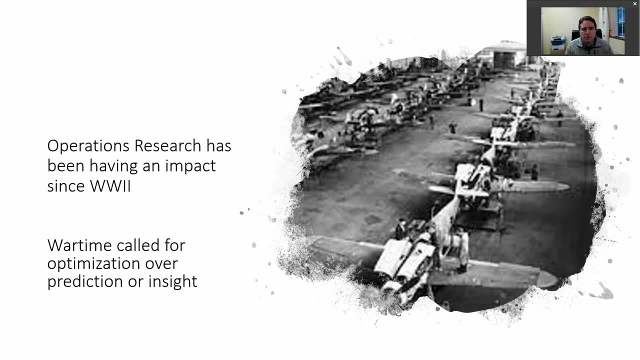 But operations researchers and statisticians have been at this for at least 80 years and had a fair bit of success improving operations. so perhaps we can learn from our ancestor field. British scientists drafted into the war effort in World War II founded the field of operations research. 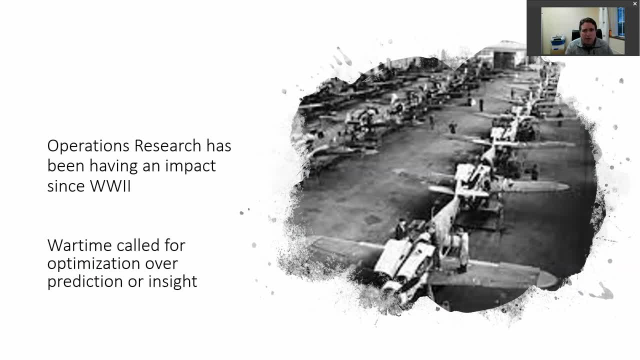 Patrick Blackett, one of the first and foremost practitioners, explains how the scientist can encourage numerical thinking on operational matters and so can help to avoid ruining the war by gusts of emotion. And indeed it was useful. Blackett helped the war effort in numerous practical ways, from optimal bombing strategy to bomb site design. 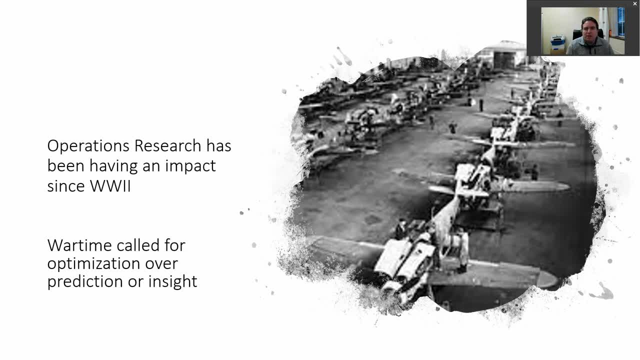 OR's first major success was Albert Rao's analysis of air defences. that led to the development of radar, key to winning the Battle of Britain. The first OR, people used to focus on the wartime economy as well. so how do I allocate steel between aircraft and girders for buildings, for example? 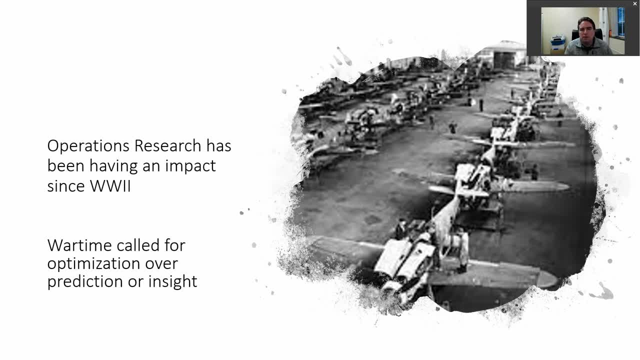 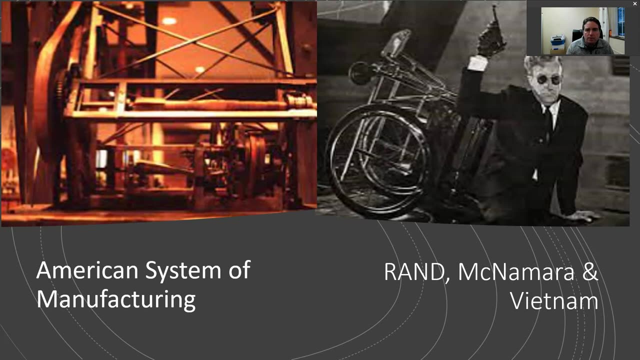 So basically, how to win a war and keep civilian infrastructure standing at the same time. While scientists had always created innovations for the economy, this was somewhat new. This was scientists directly analysing operations in the real world. Corporate America understood the possibilities and OR provided the analytical backdrop for the ultra-successful American system of manufacturing in the first half of the 20th century. 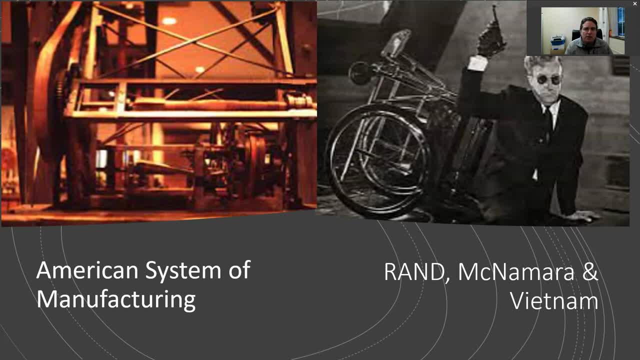 We also saw the misapplication of analytical techniques from OR and economics by Robert McNamara and the RAND Corporation, who prolonged the war in Vietnam with their dubious calculations From its inception operations. research couldn't afford the luxury of generating insights without offering prescriptions. 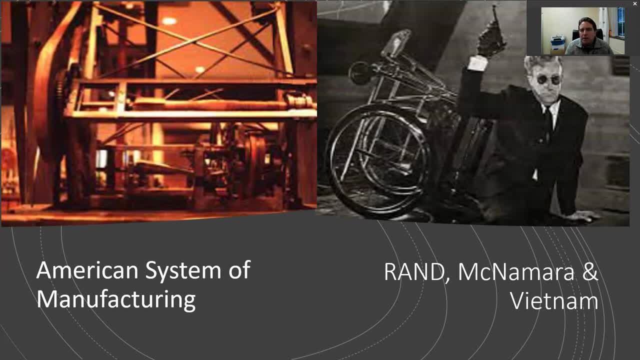 To say General, we can predict how many aircraft we will need next month, solves one problem. to create another. The General's factories tell him he can only produce so many. and what about ships and guns and other things? General, we factored in resources, demand and competing demand. This is how many aircraft we should produce next month. 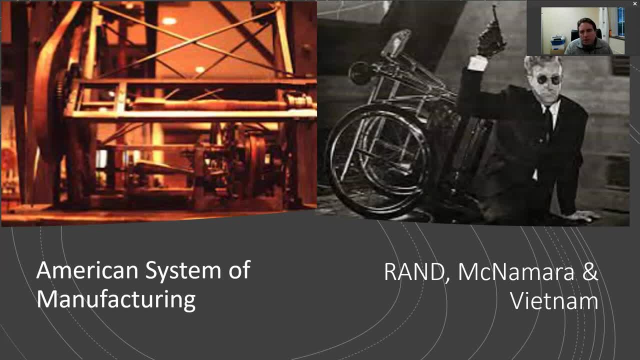 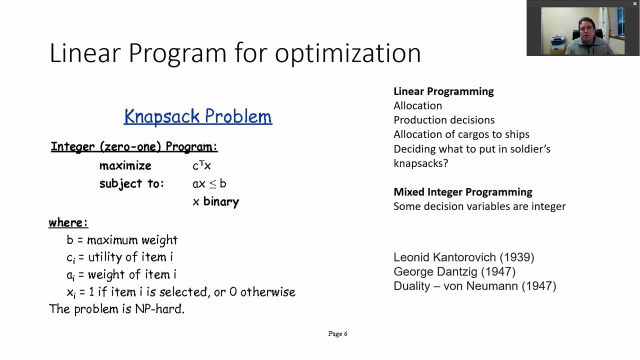 Is, on the other hand, useful. So optimization became the central preoccupation and subfield of operations research and remains so, for very good reason. It helps to get things done. Many optimization problems boil down to making the right combination of choices to form the best or optimal decision. 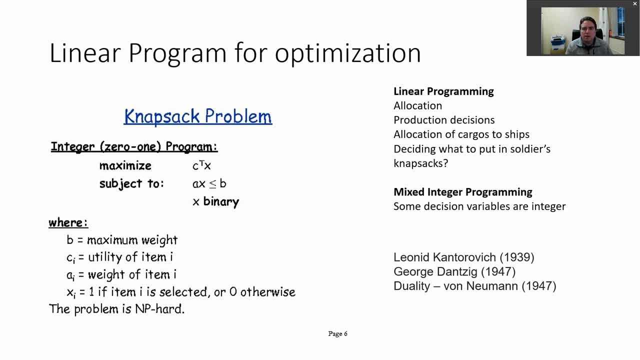 Linear programming is the classic way to represent and solve these types of problems. The techniques predate World War II, but they now got great use: Industrial production, allocation of cargoes to ships- there was no end of difficult problems to solve. Dan Sing invented the simplex method in 1947 to solve linear programs. 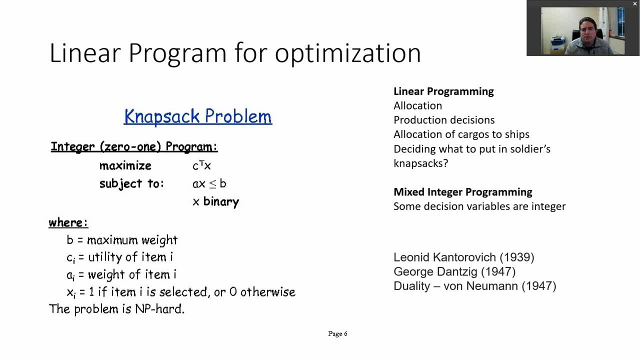 And von Neumann, while he wasn't dreaming up artificial intelligence, contributed discoveries. So what is a linear program? It's the representation of a combinatorial optimization problem in this form. So we have an objective to maximize or minimize, such as the value of goods in a knapsack. 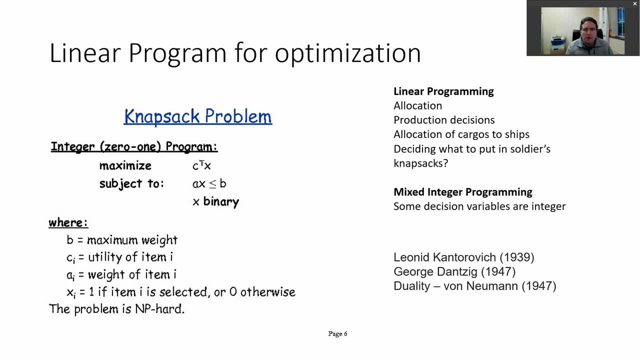 We have constraints such as the market price. We have constraints such as the maximum weight in the knapsack. We provide parameters to the constraints, such as known weights of items, And we look for the decision variables that satisfy the constraints and optimize our objective. 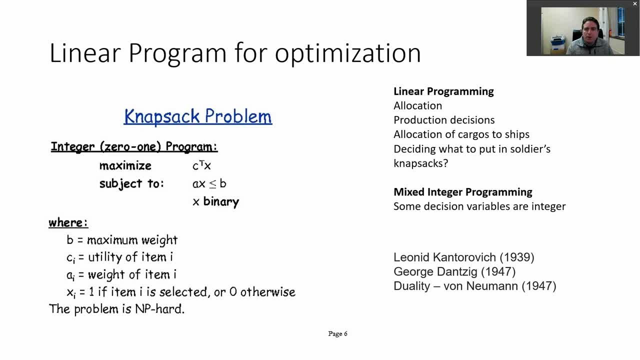 It turns out that an awful lot of business problems can be expressed this way: Where to install the first batch of 5G cell towers? How do I best use my production capability across my product range? Where should I allocate efforts to decarbonize my business? 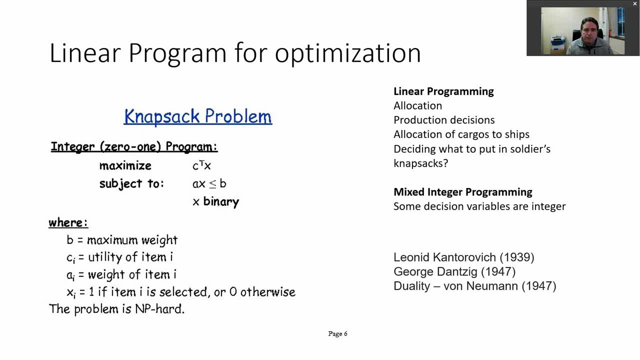 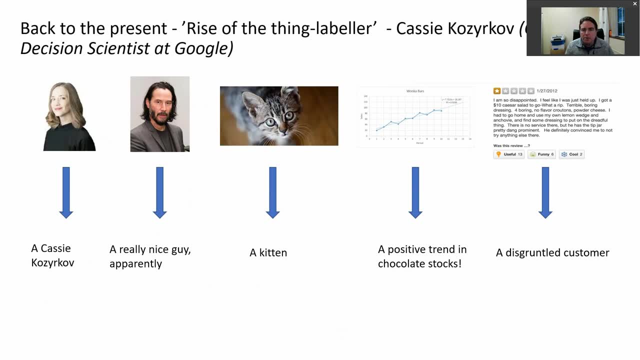 Pretty useful. I'm sure you'll agree. So back to the present, and supervised machine learning is the major AI breakthrough into industry. I won't belabor the history, as I'm sure this audience is very aware of it. As Kazi Kozakoff, head of decision science for Google, puts it: supervised ML is a thing labeler. 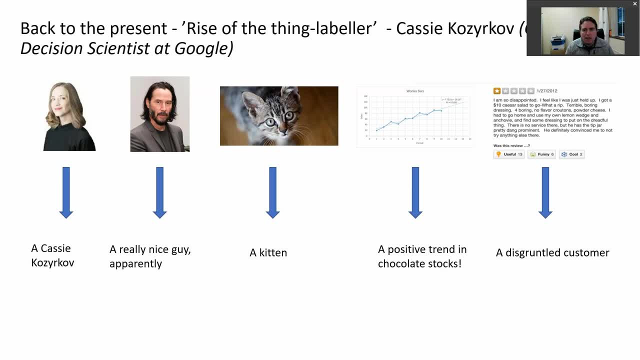 Well-trained models can predict labels for people, personality, animals, market trends, customer sentiments. So the things can be physical, like images, or abstract, like historical data. The thing- labeling- sounds kind of mundane, but it turns out that it's a key workhorse of human intelligence. 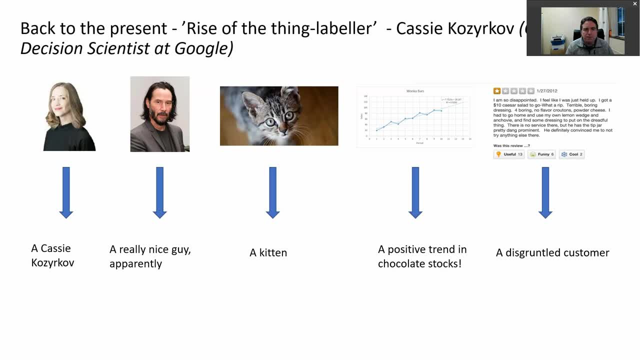 And we've just figured out how to make computers do it for us. It's huge, But what to do with these labels? If you find a lump in an X-ray, the action is obvious: Flag it with a specialist. But how do you use the labels learned on this slide? 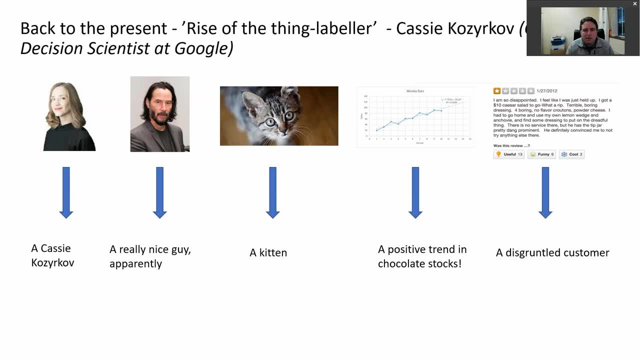 Now check if that photobomber in your holiday snap might actually be the head of Google decision science. Become friends with Keanu Reeves. Generate an alert every time someone posts a picture of a kitten on the internet. So supervised ML does an awful lot for us. 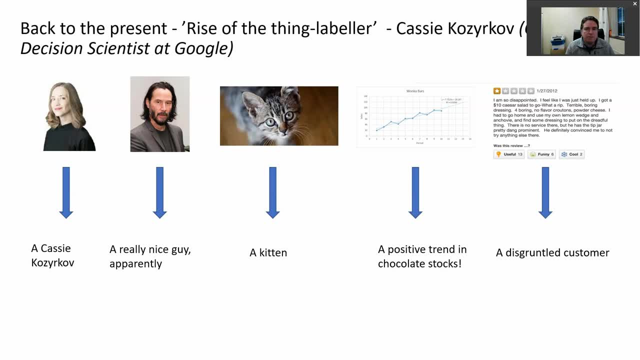 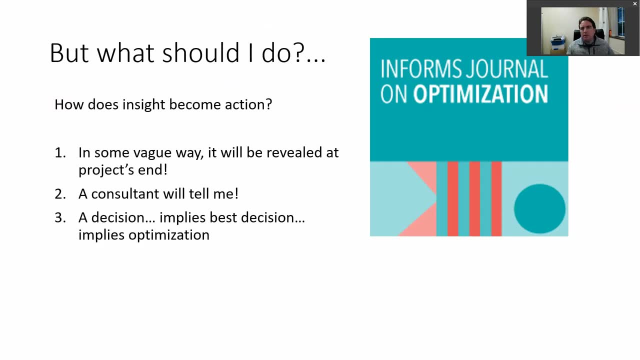 But in many situations it just doesn't give us any clear course of action And without that it's a white elephant In the real world of real deadlines and competing demands. we want to know what should I do Now? we hear a lot in data science these days about moving from predictive to prescriptive analytics. 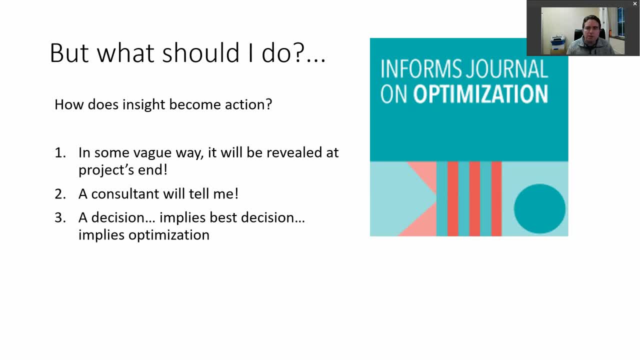 But the how is often unclear. In my experience, I've seen people clutch at two rather vague possibilities. Firstly, let's just figure it out later when we have our labels. Secondly, whoever is telling me this AI solution will surely tell me at some stage. 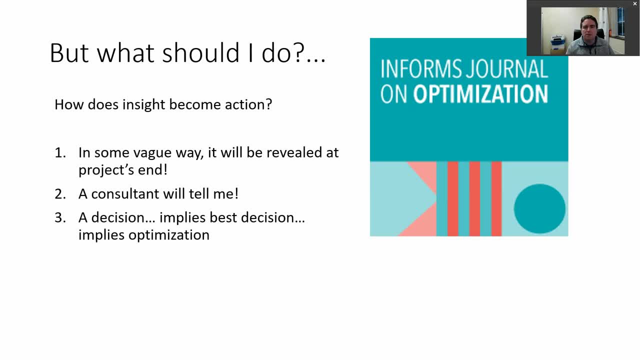 In reality, decision implies best or optimal decision, which implies the need for optimization, And we've just seen that operations research has made optimization its core competency, So we shouldn't be surprised if it is something to offer us here. It's even got its own journals and everything. 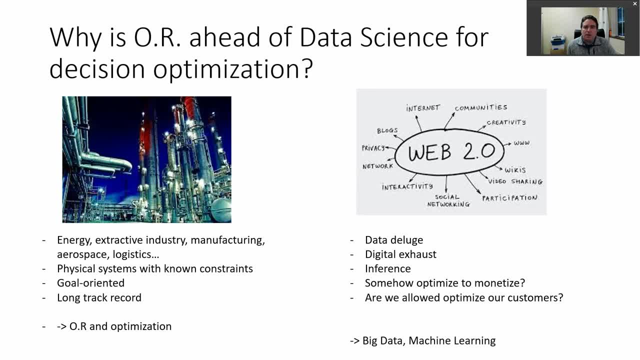 So why might OR be ahead of data science for optimal decision making? Well, I think it's down to the environment at birth. OR, as we've seen it used in the military or in primary and secondary industry, has degrees of predictability. 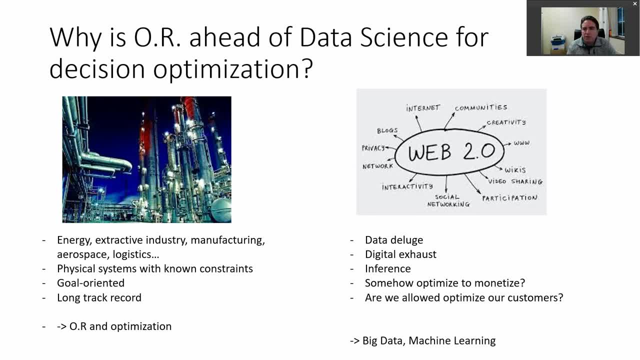 So inference is not essential. The objective, functions and constraints can be established and agreed without a lot of controversy. So no one thinks that a piece of cargo unshown for a container is going to feel left out And its users. captains of industries are all about the bottom line. 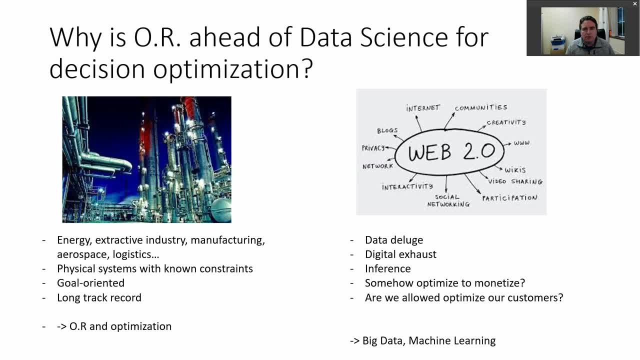 So prescriptive analytics based on optimization is really central to OR. Data science, on the other hand, has come of age with Web 2.0. in the online social world. We have a data deluge on the computer power to sort through it. 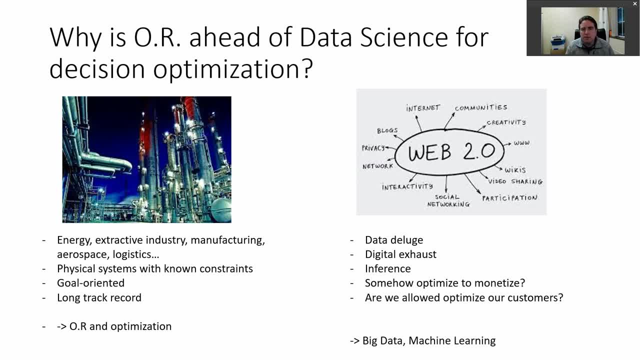 So the data is the digital exhaust from our online lives, And inference is the tool of big tech to somehow master these data streams. Optimization has been a secondary concern, generally coming later as we try to somehow monetize insights such as consumer preferences. 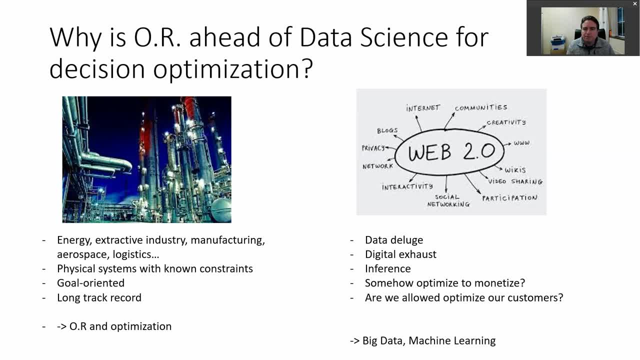 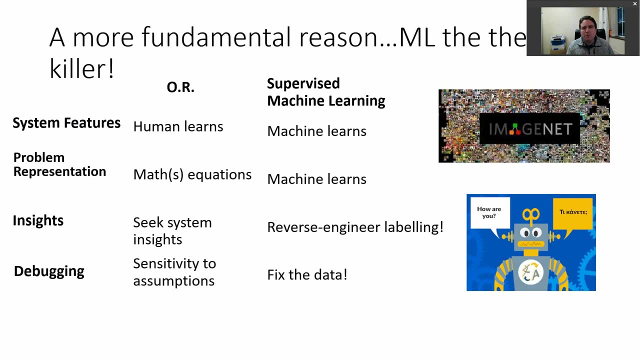 So optimization around human behaviors faces some serious ethical questions. It's not clear what is optimal for whom and who should decide. So often it's a case of better the machine learns than takes control. But there's probably a more fundamental reason. 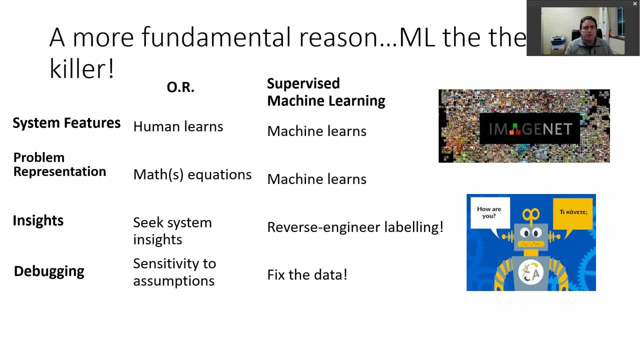 OR seeks to understand complex processes And maps them into a formal system for solving. In doing this, we uncover essential attributes of the system, including what is valuable, what is possible, what is not possible. Although the techniques are generic, the model of each new situation is entirely different. 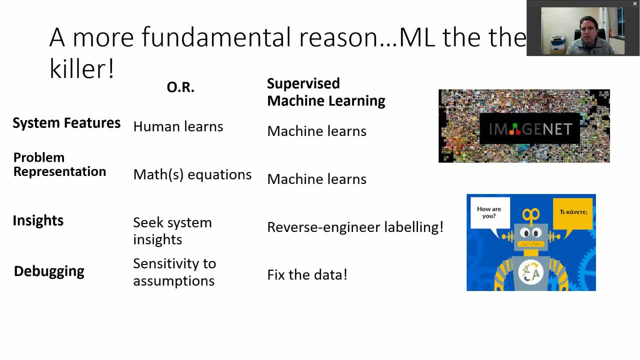 On the other hand, ML seeks to apply a metamodel to generic problems such as image classification or machine translation, And I don't think I need to tell this audience that it's been wildly successful in this. Alex Krizewski's AlexNet won the ImageNet competition in 2012,, beating out experts in computer vision without having any background in the field. 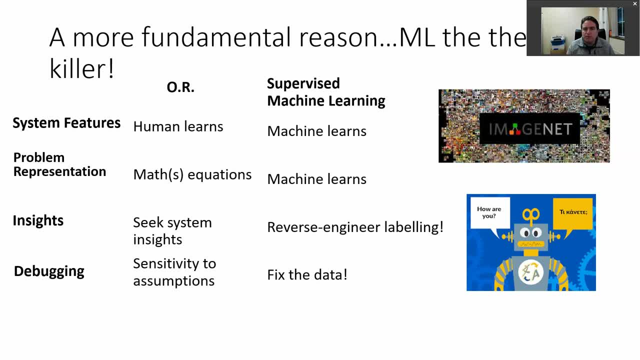 Neural machine translation is outperforming linguistic models painstakingly put together with decades of research. This is the great power of machine learning. and now deep learning. There is this incredible orchard of low-hanging fruit where we can do what seem to be highly complex very easily. 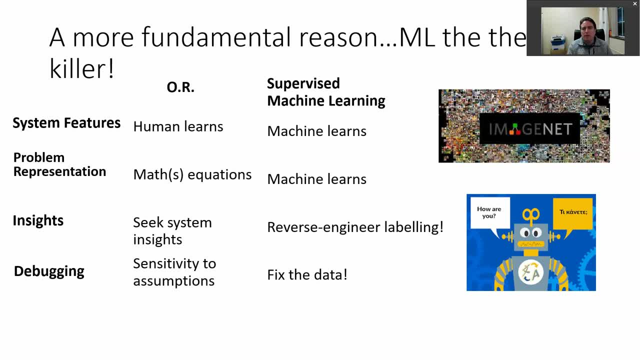 And I for one, have no problem with this at all. So one of the main areas I work in helping companies is using ML to kind of reap that low-hanging fruit, And the translation into business impact is still not trivial. So there's plenty for us all to do. 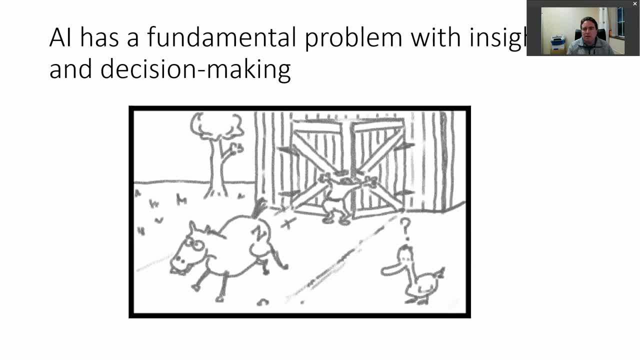 But here's the thing. The promise of deep learning is that we can master a system, whether it's widget production or fraud detection, without truly understanding the system. Where does that leave us with decision making? Well, it's hard to make a decision. 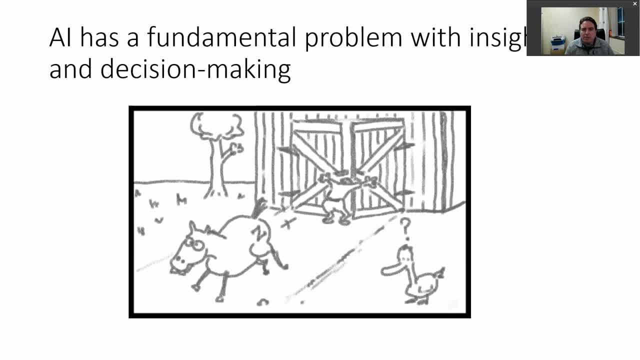 Well, it's hard to make a decision from an inference about a system when you fundamentally don't understand the system. Yes, there's a lot of work going on on interpretive AI and causality at the moment, But I see hard theoretical limitations on trying to reverse engineer labeling systems to generate the kind of insights that support complex decision making. 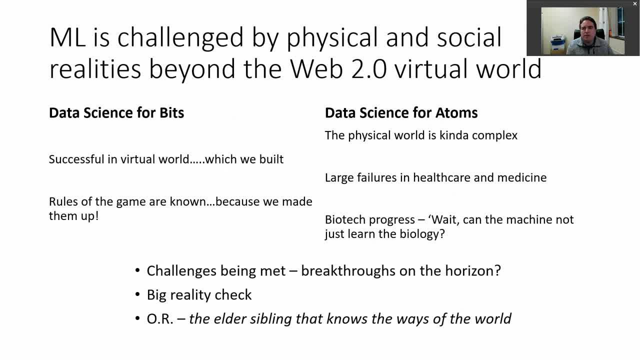 So what do these limitations mean in practice? How is data science doing at the moment? Well, in one sense, data science and applied ML have been hothouse flowers doing very well in their own environment. But, as Peter Thiel has complained, tech has not progressed in the physical realm of atoms as much. 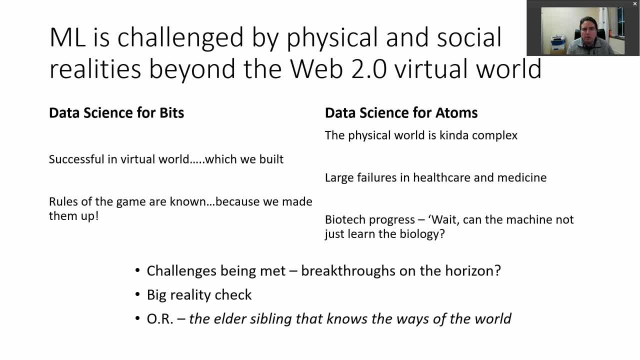 And there have been some spectacular Silicon Valley failures in bio education and health over the last decade. Now, in the online social world, programmers constructed the online platforms, So it's very easy for them to understand and manipulate people's behavior on them. 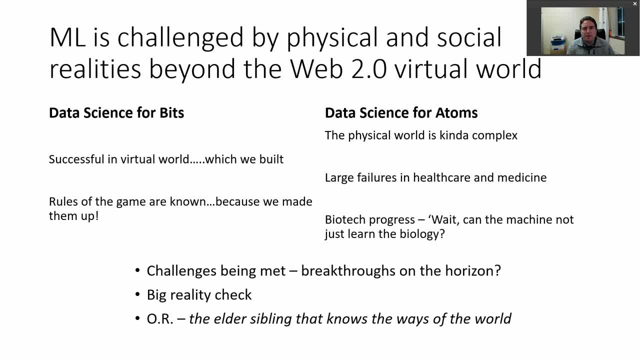 But as we move out into the real economy, we are faced with some very complex physical and social systems. The big takeaway from the biotech revolution so far seems to be: better start cracking the biology books, better understand the system before applying ML. Now these challenges are being met and serious leaders in the field like Andrew Nung, Drew Conway, Henry Mason and DJ Patil are now grappling with complex systems: health care, energy, education. 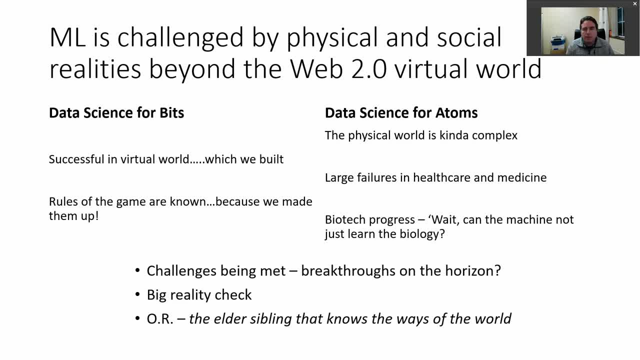 But the move out into the real world has been humbling for the field, So maybe it's time to lean on the big brother or sister that is operations research. They've been living out in that world for quite some time now. Of course, it's not an either or for ML and operations research. 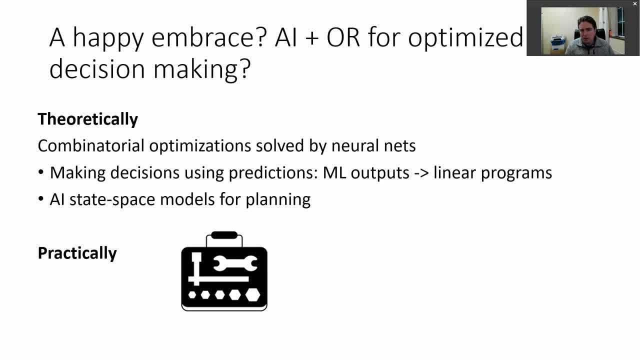 There'll be a relationship between them. We're starting to see, for example, ML used in place of OR for optimization, But I do think this is hard limits and interpretability, as discussed before, And some companies, like Stemly, who I do some work with, are starting to close the loop. 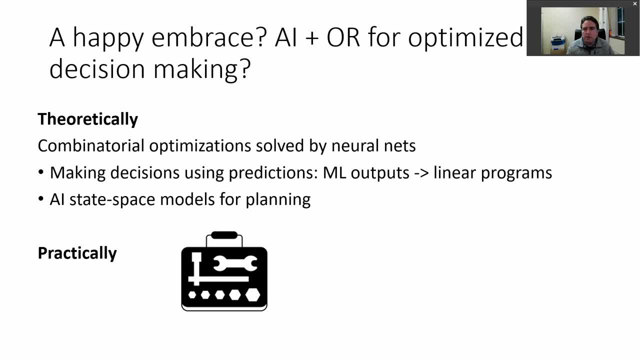 It's very interesting. It's a hybrid ML and optimization solutions, And AI itself has a lot to say about production planning, for example. Even within ML, we're starting to see use cases for reinforcement learning from multi-step optimizations, where we can model agents. 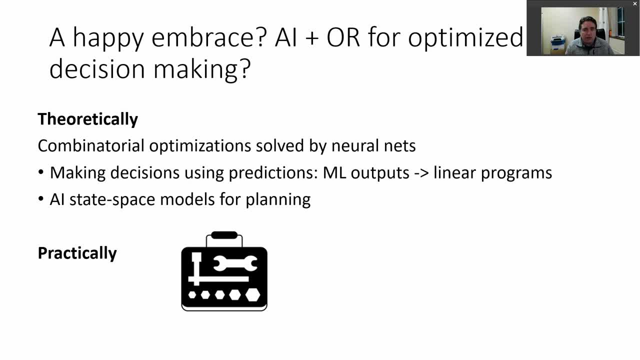 But the subfield of AI for planning has been active for decades and has had successes in industry. In the standard reference for the field artificial intelligence by Russell and Norvig, the first half of the book covers planning theory, But it doesn't make an appearance until page 693.. 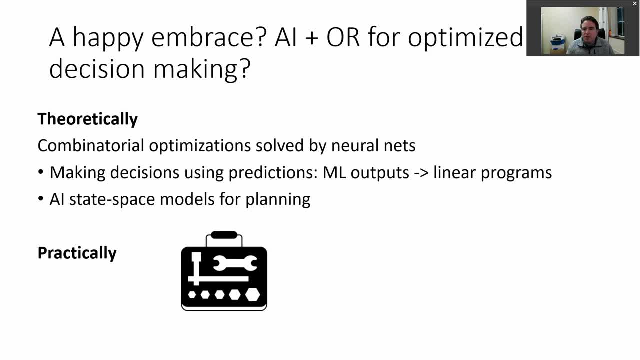 So it's the ultimate suspense thriller in that regard. So it's not an either or in terms of AI and optimization, But with my practitioner hat on, I see the clear and immediate benefit of embracing OR. It adds another perspective and set of tools to our data science toolbox, especially for optimized decision making. 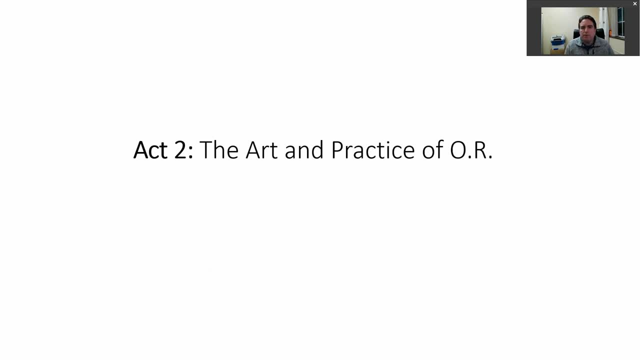 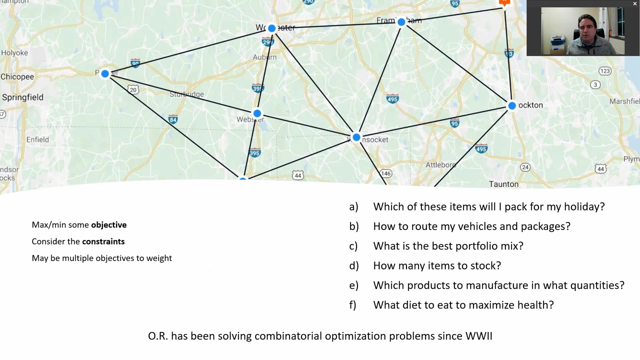 OK, so hopefully I've convinced you why a second look at OR could be of value. So what does that mean to us in practice? How does OR help us conceptualize and solve problems using a computer and some software, particularly Python software? So OR has been solving NP-hard problems for decades now. 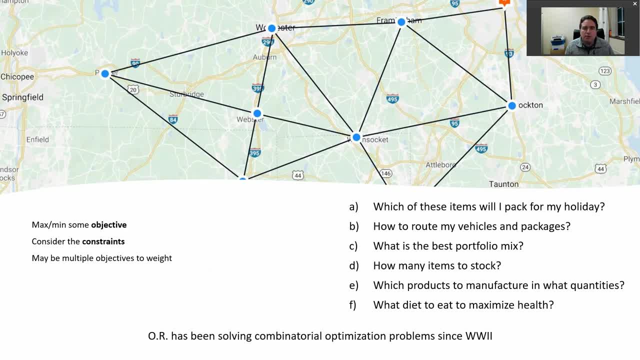 Consider the traveling salesman problem: to find the best route to take through multiple cities in a sales trip. Now what is the combination of cities to choose to form that best route? Best could mean cheapest or fastest. We might have some constraints, such as visit all cities. 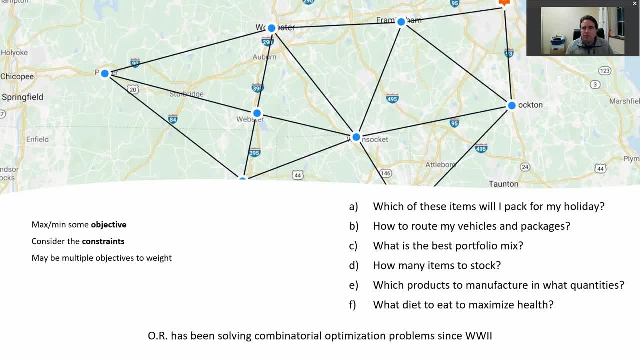 Visit at least half of cities. Don't visit any city more than once. We might insist on returning to the start point at the end, or we might not, But ultimately it boils down to the best route, the best ordered collection of cities. 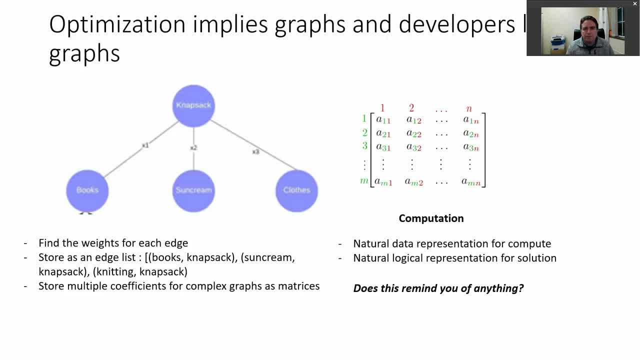 So it's a combinatorial optimization problem, And you may have noticed that the TSP can be represented visually as a graph. It turns out that all combinatorial optimizations can be, And, of course, graphs are not just visuals, They're a representation of a system. 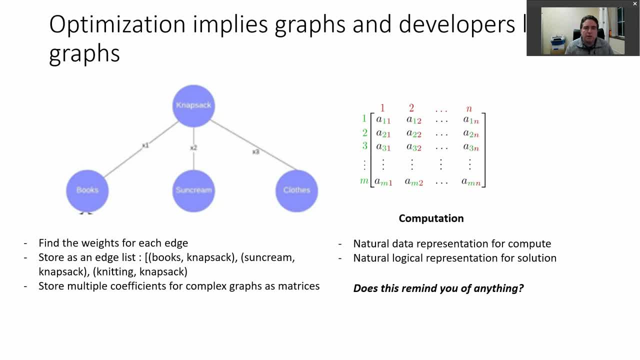 With some very nice mathematical properties and techniques developed to work on them. In computer science we can store graphs as very efficient data structures And all sorts of tools to manipulate and query them, For example, shortest path, minimum spanning tree, and so on. 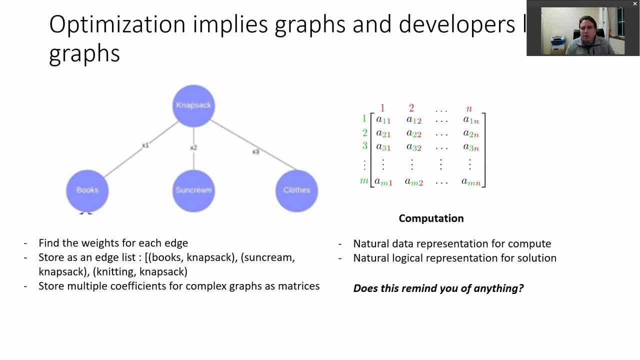 So let's take this example of the knapsack problem, Where we want to know how many books, sun creams and clothes to take on our holiday. What we really end up looking for is in this diagram here, x1 to x3,. 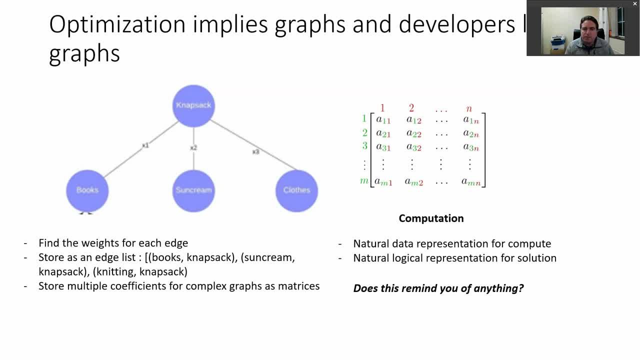 the values to assign to each of these items that we're going to take. So what we're really going to find is the value for the edges in this network Or graph. If the graph gets more complex, we can store all these layers in a multidimensional matrix. 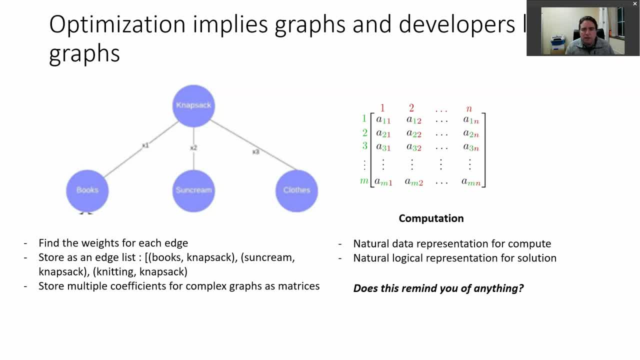 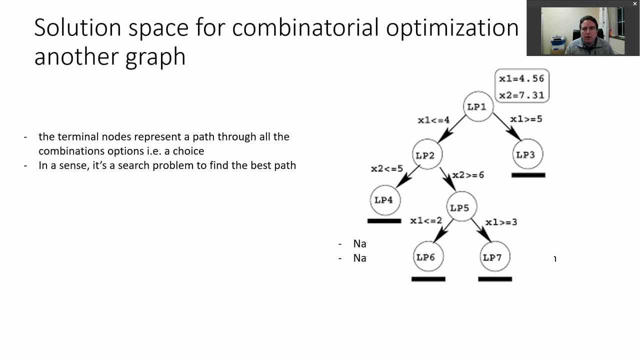 Where the indices stand in for the vertices we're connecting. If anyone has worked much with machine learning, this matrix representation should start to feel very familiar. The solution space for combinatorial optimization. Combinatorial optimization is yet another graph, So the terminal nodes present a path through the solution space. 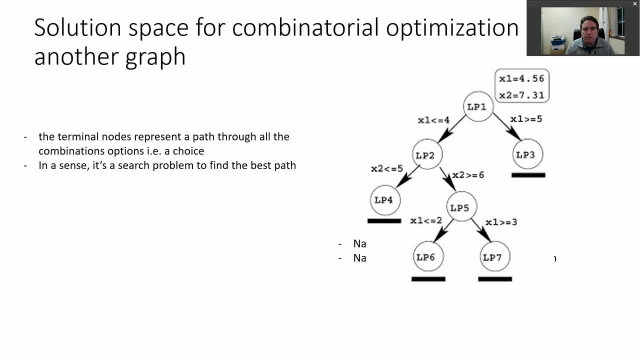 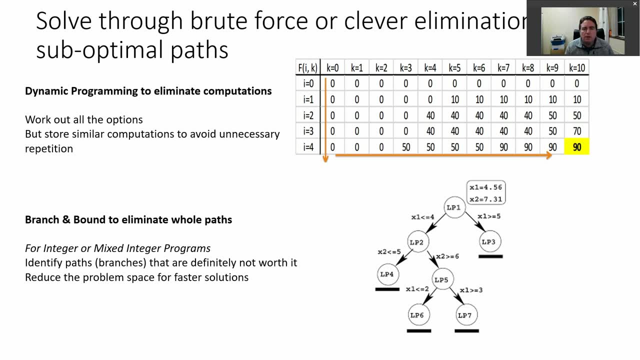 In a sense, then, it's a search problem just to find that best path. So again we're in classical computing land. We can just go ahead and exhaustively search to find the optimum solution, And dynamic programming is a perfectly reasonable way of doing this. 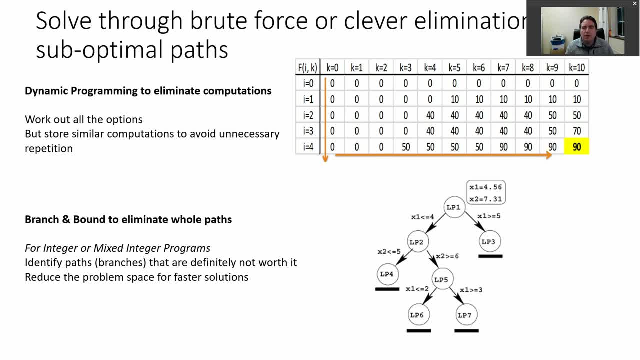 We don't save on search costs, but we make sure to store similar computations to avoid unnecessary repetition. Or we can be cleverer and use algorithms developed in OR to start eliminating options and reduce that search space. Branch and bound is the classic algorithm here. 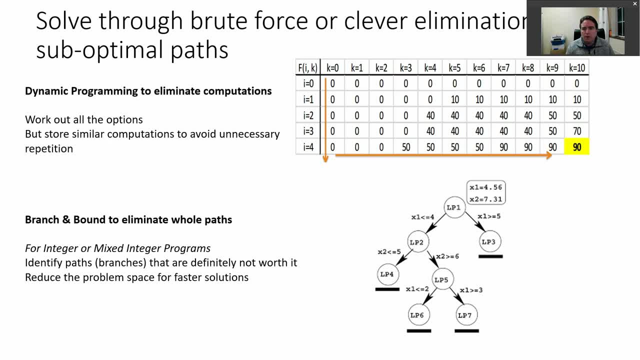 We can think of branches as sets of possible solutions. Before we exhaustively check a branch, we can establish an upper bound for the best solution And compare it to what we already have. If there's no possibility of the branch giving us a better solution, we can just disregard it. 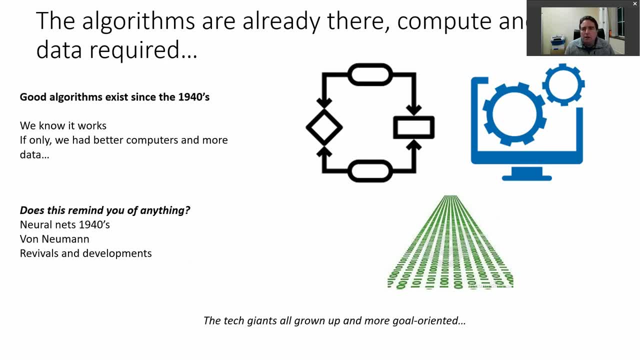 And we've many advancements in algorithms since branch and bound And, as with any established algorithms, people have worked out efficient implementations in software, so you don't have to. You can usually leverage a library to implement this part, once you set up the problem correctly. 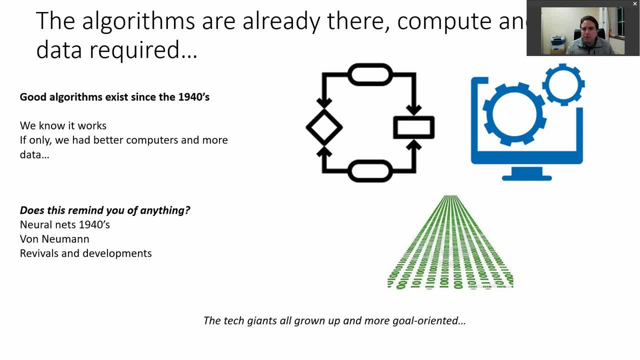 Now, because we're dealing in combinations, runtime increases exponentially with the number of variables. So one of the issues we face in OR is the computational complexity remains high, But with Moore's law on access to cloud compute we're seeing speedups that make it possible to run heavy optimizations in batch windows. 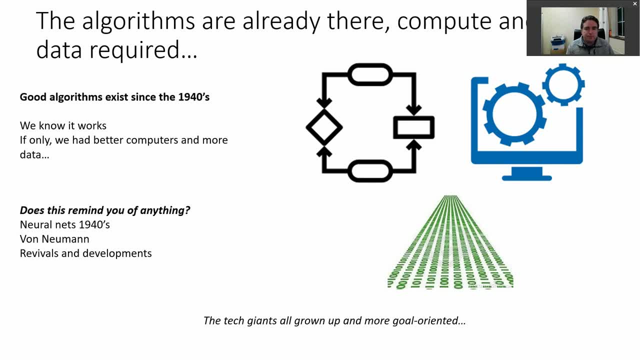 or even in near real time behind web applications. So I wonder, does this remind you of anything? Not anything at all. We had neural nets since the 1940s and had to wait for better compute and data access to take advantage, And in fact von Neumann was involved in the birth of both fields. 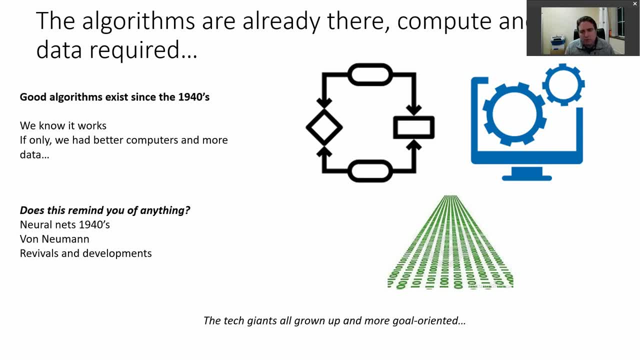 Of course he would be, And now we have the data science world much more focused on optimizing against goals. So in practice, taking a new look at OR seems timely for practitioners. One of the interesting questions I've had from data scientists and optimization projects is: 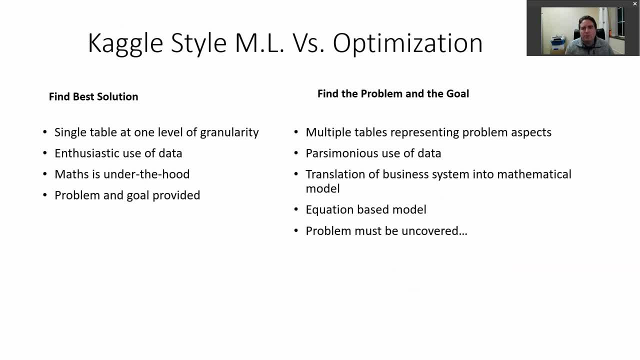 where's the table And how to answer. which table? So you need: the one to use for the production constraints, the one for inventory parameters, the one for goals. So when we model an optimization, we can work on various levels of the problem. 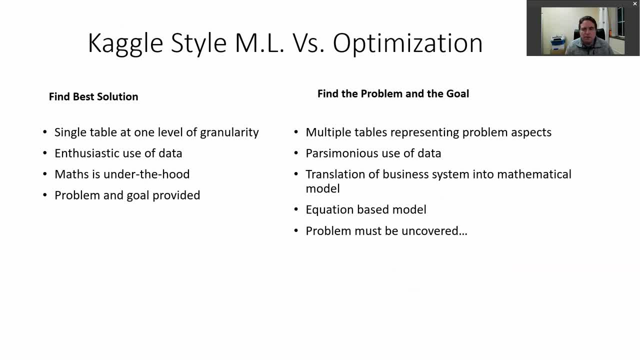 Each level of the problem will require a table or set of tables, often with different granularity. This is very much in contrast to supervised machine learning, where we tend to, in the end, line up the data into a two-dimensional matrix or table. 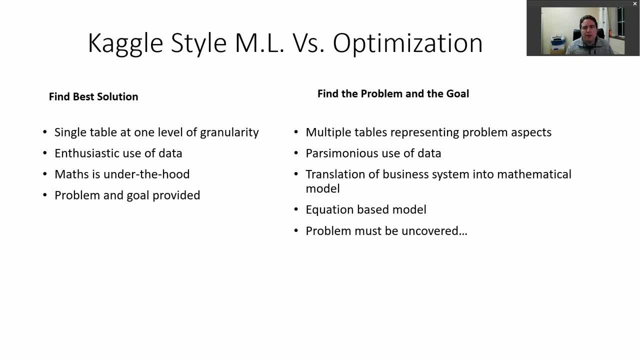 Now the compute for deep learning is very complex. The compute for deep learning is very much dependent on the number of records and features, that is, the size of that input table. The more data, the better the model performance, but the worse the code performance. 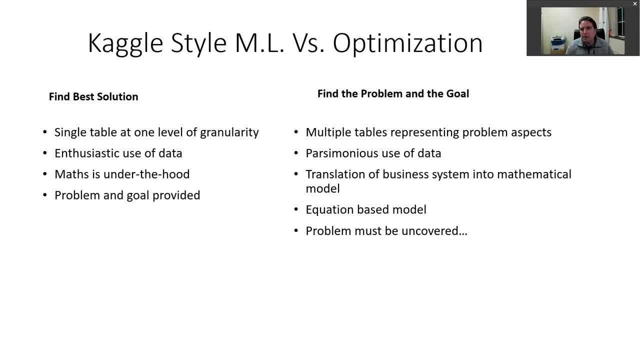 With optimization the data can be tiny, but the order of complexity is not based on that. Rather, it's based on the number of possible decisions, the search space. You can easily generate a solution space with 100,000 variables from a few small tables. 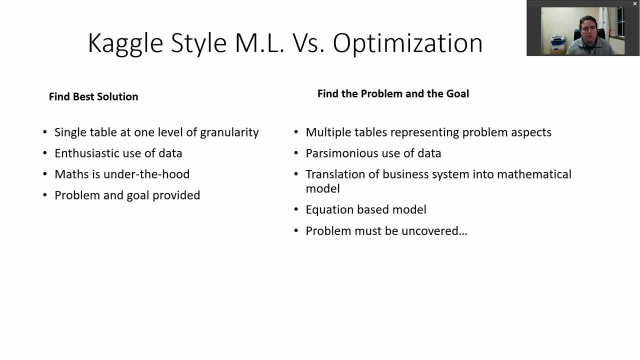 and a complex set of constraints, So the compute time will rise accordingly. It also needs quite a bit of work to process the data into the right shape for the problem, probably more so than for ML problems, where the only designation possible for a piece of information is a feature or a target. 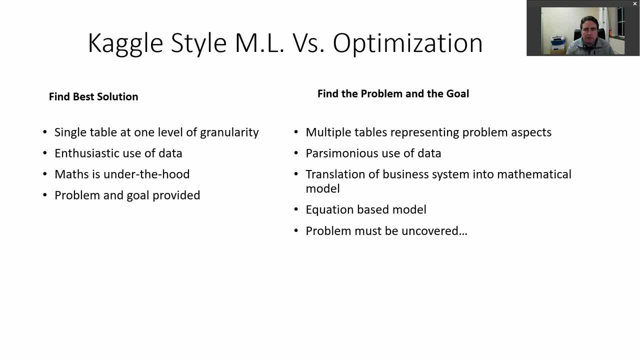 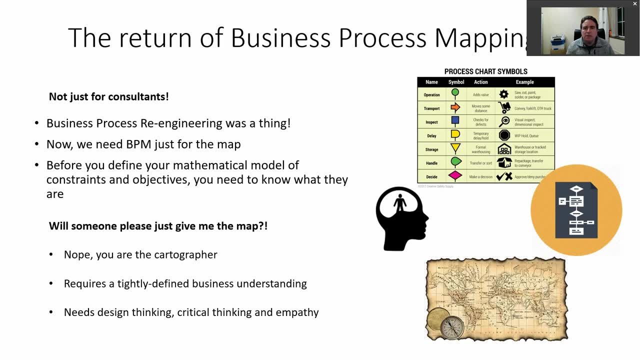 As we'll see, there's a bit more analysis and mathematics involved as well in setting up an optimization. Now, back in the 1990s, every consultant in the land wanted to map and re-engineer your business processes. Well, this is actually necessary for defining an optimization problem. 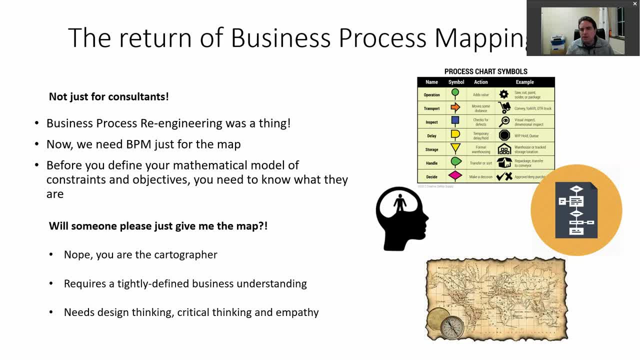 For a supply chain. what goods can be held in what vehicles? what are their capacities? loading and unloading times, maximum travel distance per day. what does the network look like? what nodes can be linked? what cannot? what about delays? 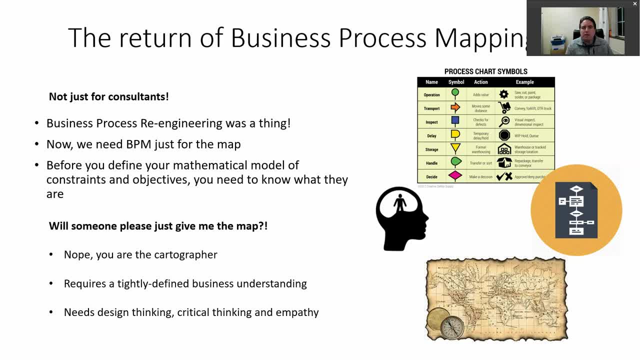 If we're trying to minimize costs, how do we define those costs? Are they fixed or variable? Over what horizon? What service level must we reach? How is that measured? How do we cost the missing delivery? So you need to know the system precisely. 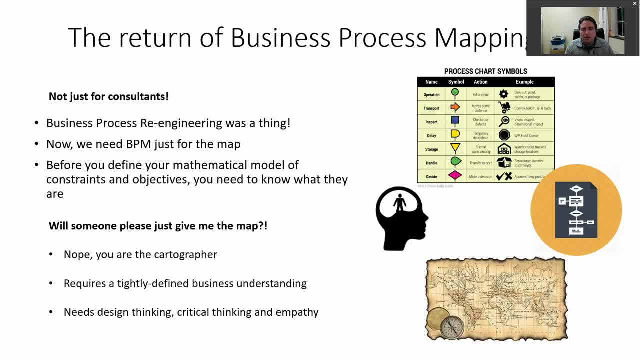 If you have any chance of turning it into a mathematical model. So how do you get this map? Ask the client. You may find this weird. for anyone who hasn't worked in business for, say, a long time is that most businesses do not know how they run exactly. 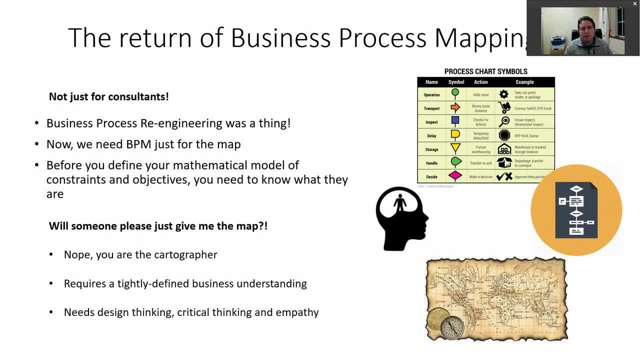 How operational processes arise is very organic, and the knowledge is held in various brains dotted around the organization, So be prepared to learn a whole lot about chicken farming, ice cream, transport policy, forestry, emergency health care, renewable energy or whatever industry you're interested in working in. 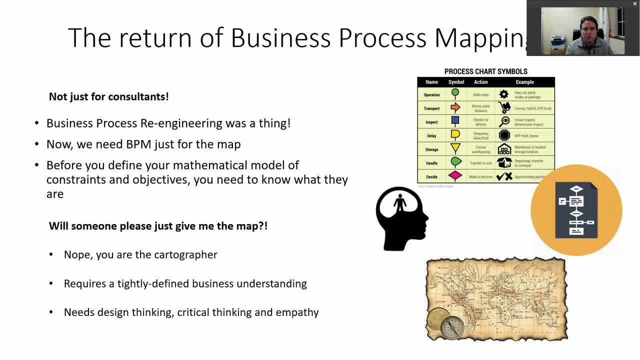 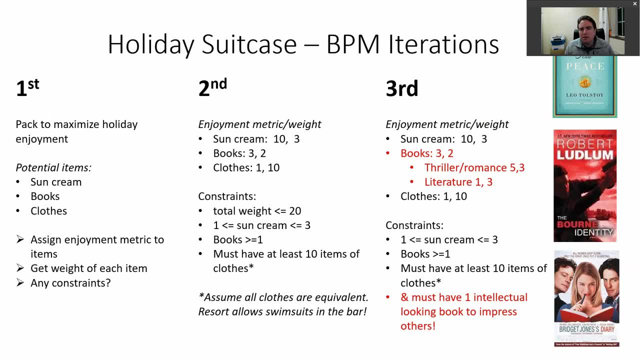 This is the great pain and sometimes the great joy of operations: researching the operation, So mapping a business process, means making those key details explicit. So take the example of packing a holiday knapsack or suitcase. Let's say we can only take sun cream, books and clothes. 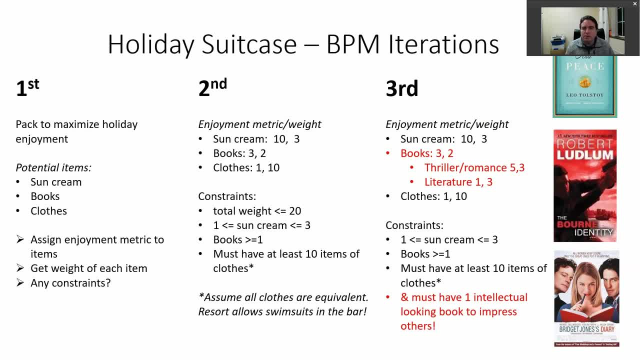 We'll need to assign some kind of enjoyment metric to items, get the weight of each item and then apply constraints. So in our second pass we find that we need to maximize enjoyment up to our 20 kilogram limit for our items. We might have other constraints. 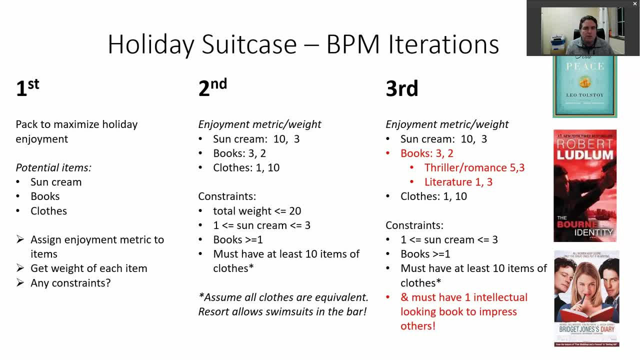 For example, I need at least one sun cream, one book and 10 items of clothes, But more than three sun creams would be not very useful And we have to assign our parameters. So weight is easy. We can get the weight of these items. 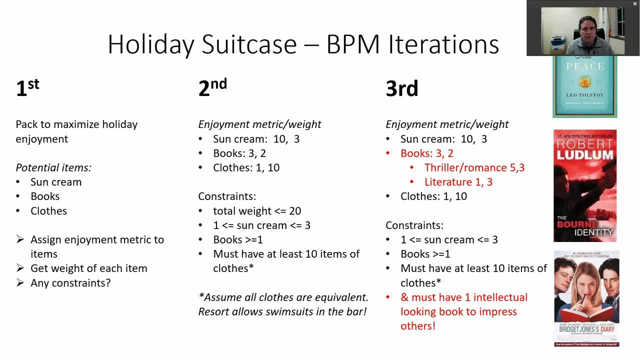 But the enjoyment metric might be quite difficult to apply across these disparate things. So we come up with those metrics And those weights. Maybe we run our optimization and we end up with war and peace and Ulysses in our suitcase and feel kind of depressed about that. 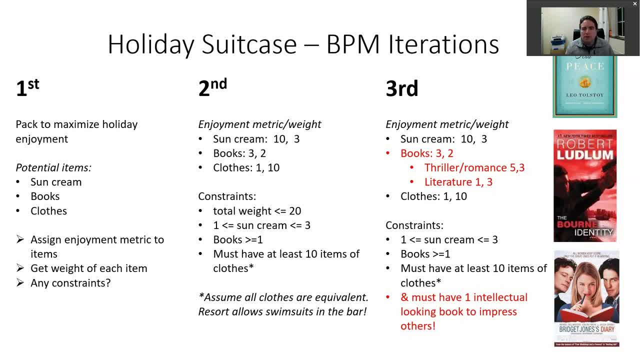 So we figure not all books are created equal. What we really want to read on a holiday is something easy and fun, As long as we have one literary work so we can say we tried. So that gives us another set of constraints and another kind of level to this model. 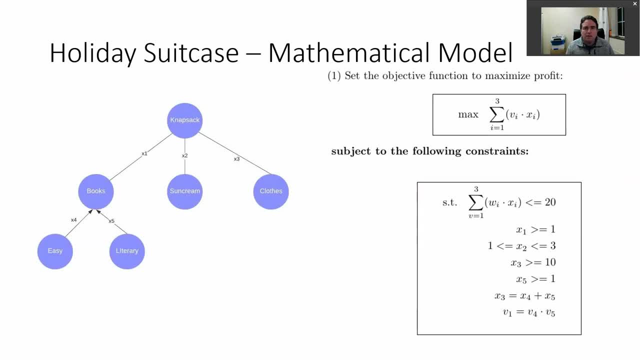 So how does that look? Well, it basically turns out to be this: It turns into a graph, just like the knapsack, but with this extra level now, So we can define books as the total inflows from the easy and the literary books. 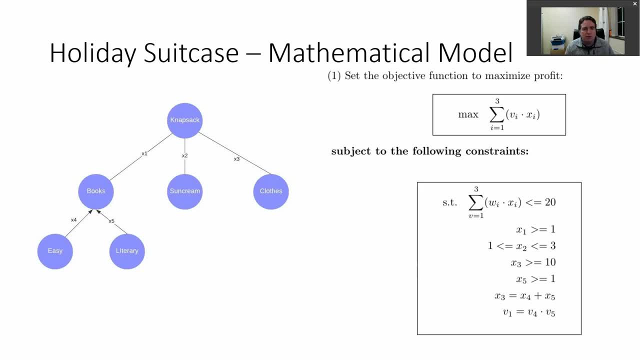 Technically, in optimization we deal with inequalities, But it's easy enough to extend to equalities. So we can make that. We can make that connection between the nodes. So what we get here in these eight equations is a precise mathematical model of our business. 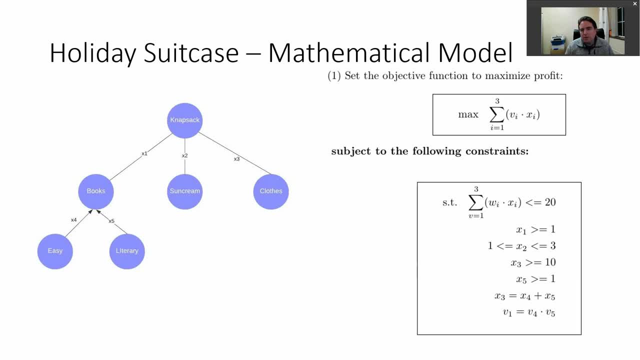 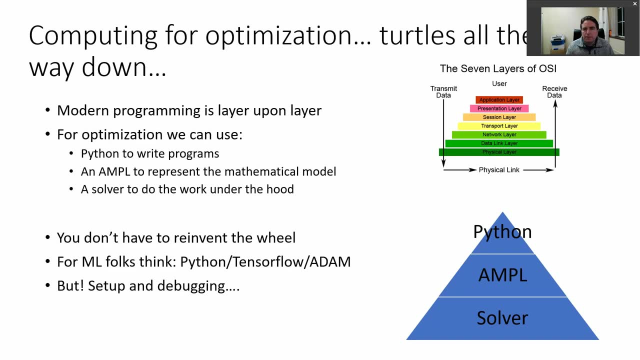 or our holiday packing process, And then we can go and turn that into a program and its data for solution in Python. Like with most programming tasks these days, we find the functionality exists across several layers. So for optimization we can use Python to write the programs. 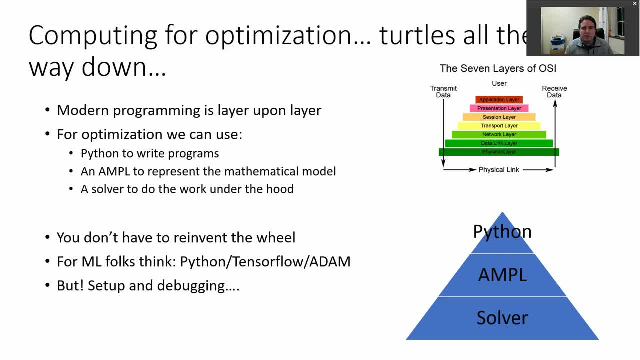 an ample mathematical programming language to represent the mathematical model intuitively and a solver to do the work under the hood. You don't need to reinvent the wheel. So for ML, folks think Python, TensorFlow and maybe add them under the hood. The only issue here is that debugging across these layers can be something of a nightmare. 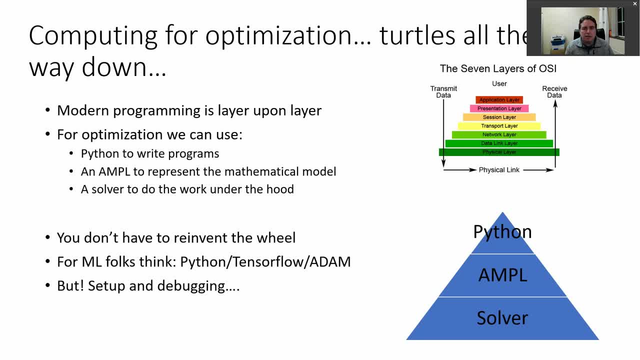 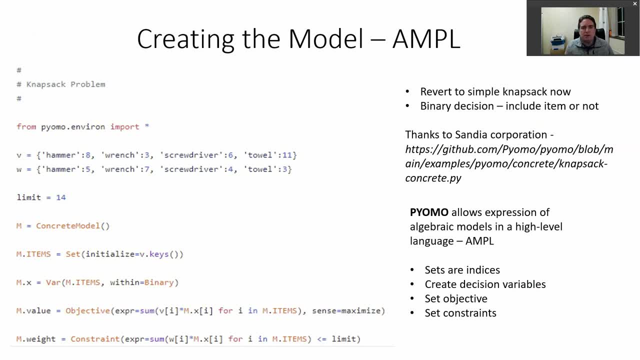 It requires some good testing practices to isolate errors, And then we can go and write the actual program using the ample constructs in Python. So this example uses the PIOMO ample. Here we refer to the simpler knapsack problem where it's a binary decision. 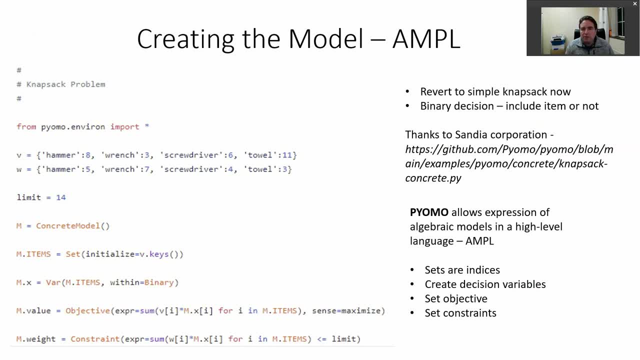 Include an item or not. We can define the parameters as Python and Python. We can create different data structures, such as dictionaries, and set other variables as well, For example limits. We then create PIOMO sets, which are indices used to keep track of the variables. 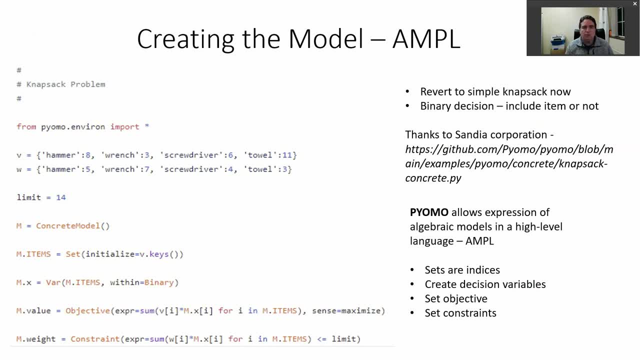 And we create decision variables for the model, In this case, which will take the values of yes or no for each item. This is a PIOMO specific data structure that will be used during the modeling run. Then we set the objective, function and constraints using mathematical notation. 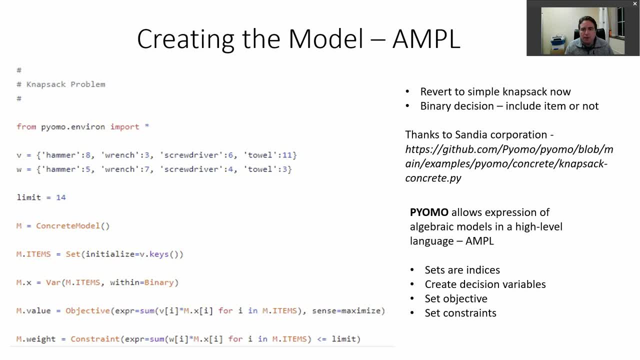 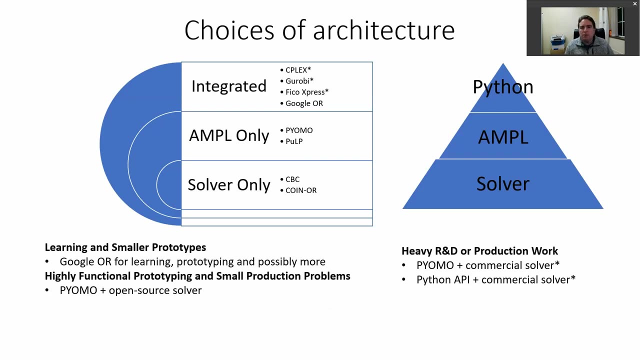 PIOMO variables and Python variables for any constants. So once you have your mathematical model of your problem and you have intermediate knowledge of Python, you can get to grips with optimization in Python within hours. Now you can use Python for tinkering around up to serious R&D and even up to production systems. 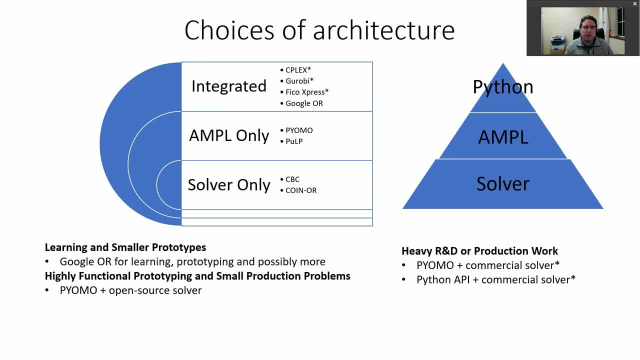 Which is very handy so you can keep all your data processing in pandas, numpy or whatever Python packages you use, and your optimization all in one code base. There's a very large choice of options here, So you can use an integrated toolset like Gorobe, Cplex, Express or Google OR. 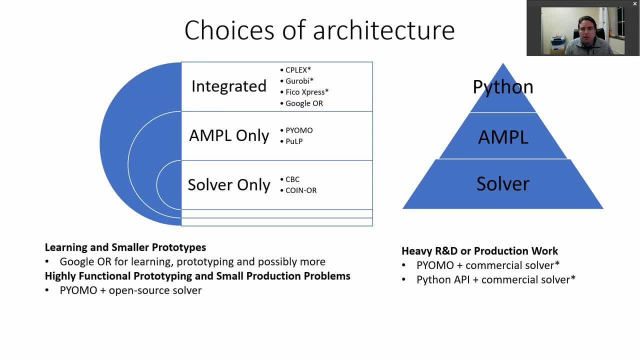 which all have Python APIs, Or you can use PIOMO or another AMPLE to interact with either a commercial or an open source solver. The difference between the commercial and open source solvers is mainly in computational efficiency, So for large problems you'll probably need to shell out the license for a commercial solver. 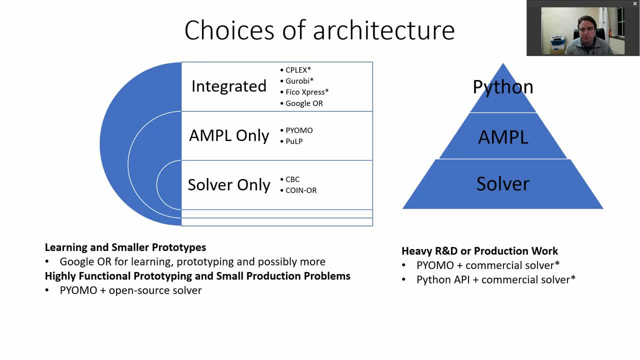 if you want them to solve in reasonable time or at all. But in terms of functionality it's all there for free with open source solvers, So that is only required if you need to scale up. One thing to note is we've been only talking about linear and integer optimization. 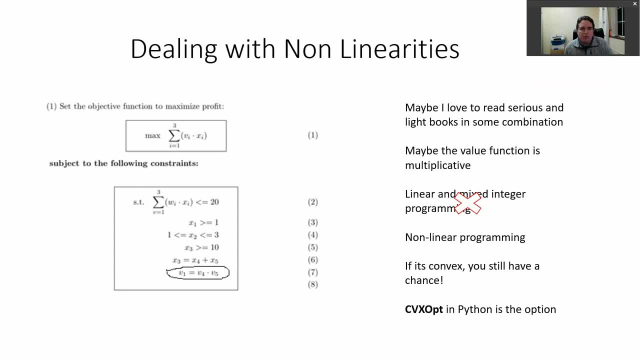 And non-linearities can arise in quite simple seeming situations. So if I love to read serious and light books on holidays, in some combination there's a dependency between those variables And maybe that value is multiplicative. At this point the problem becomes non-linear. 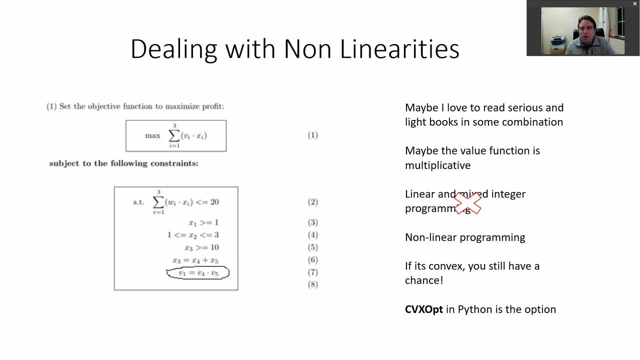 And the software I mentioned so far won't cover it. Now you can check the problem for convexity And if it is convex, you can use non-linear methods. For example, there's CVXopt and Python which will take care of convex non-linear programs. 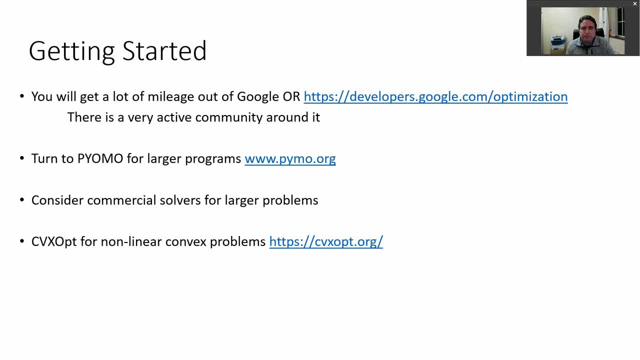 So all is not lost in those cases. So, in terms of getting started, I'd recommend to start out with Google OR. So it's a great tool with some very nice tutorials and a reasonable sized community around it. PIOMO is more fully functional. 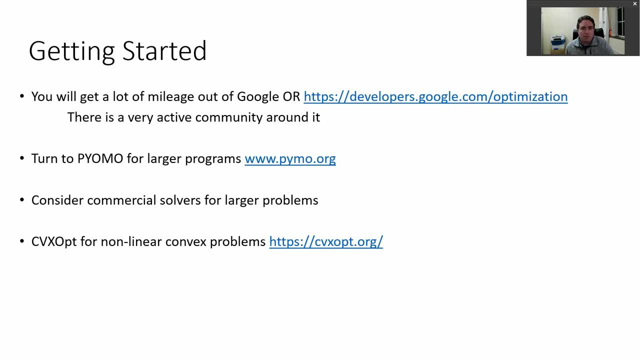 And you can use it for free with an open-source solver for complex problems. as long as the number of variables is fairly low And the commercial solvers are very powerful- And some have IDEs like iLog Studio for CPLEX- They're very much worth it for commercial heavy use. 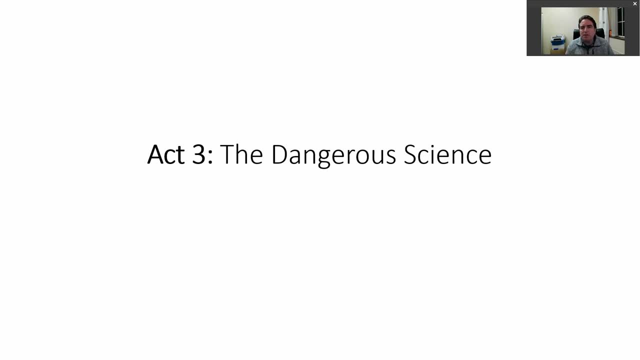 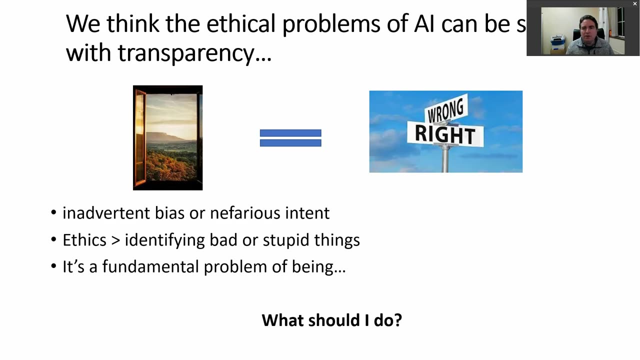 Okay. so just in case we get too happy with ourselves, let's briefly consider one pretty serious problem we're going to encounter as we start to use more OR in data science. We think that ethical problems of AI can be solved with transparency. So if we understand the hidden biases of a model, 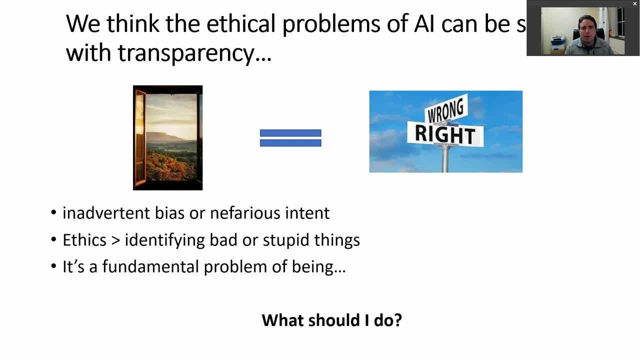 expose all the negativity. then we can get to an ethical AI. But ethics is more than identifying bad or stupid things. It's a fundamental problem of being What should I do Now? ML gives us inferences, but optimization tells us what we should do. 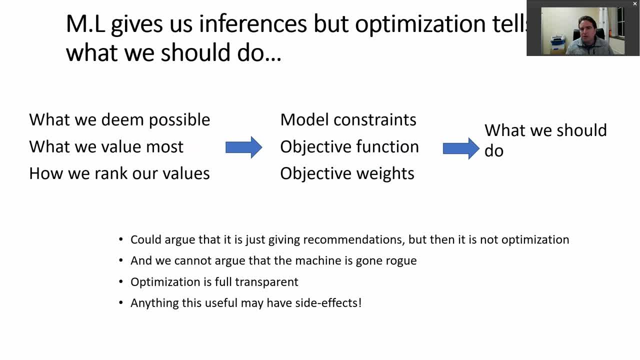 That can be a little more controversial. Optimization also asks us to search out and explicitly define things like what we deem possible, what we value most, how we rank our values. Now, emotional creatures that we are, we hate to trade off anything involving human values.